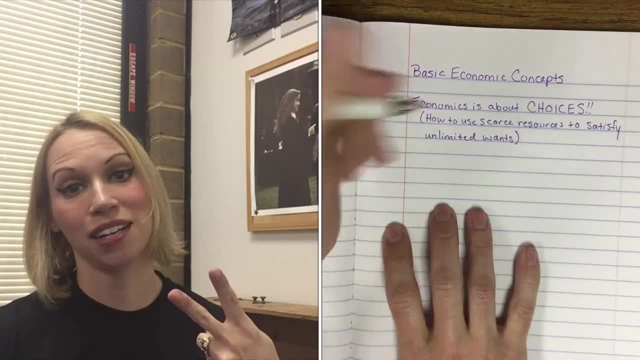 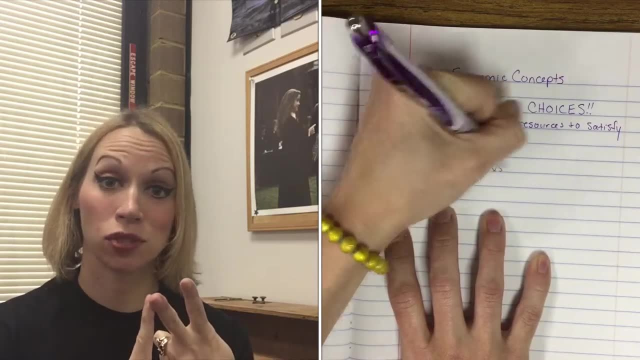 life. Now there are two branches of economics that we're going to study this year. There's going to be microeconomics, which we're going to study in the fall, and then macroeconomics, which we're going to study in the spring, a little bit later. Microeconomics means that we're going to 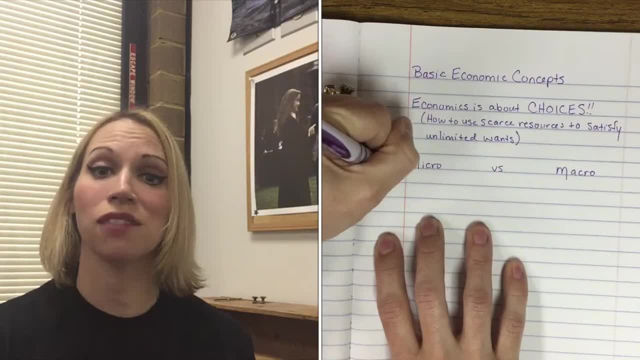 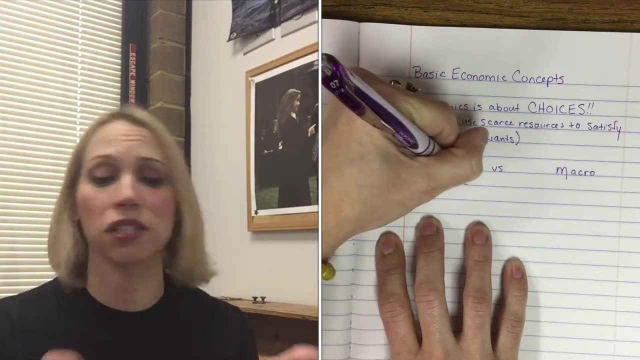 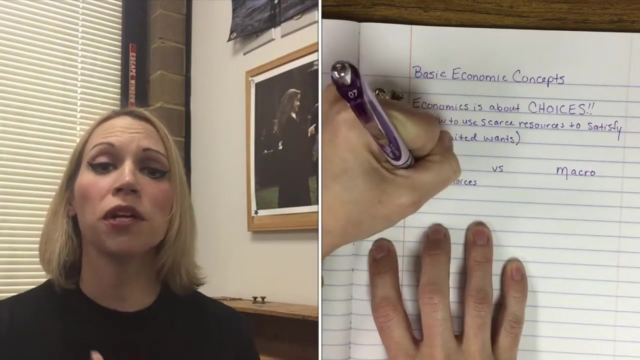 be zooming in on the individual choices and decisions of specific customers and specific businesses. So we want to know why did that customer choose this product over that product? and we want to know why did that business hire three workers instead of four workers. We're going. 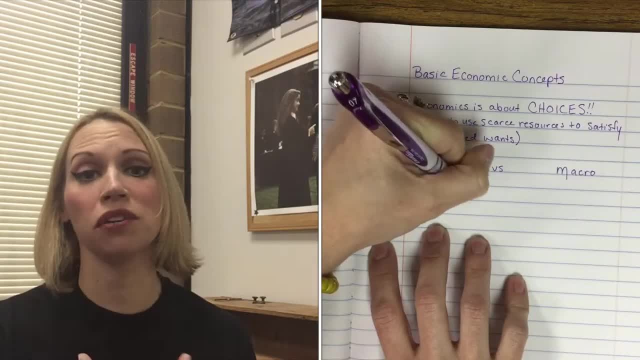 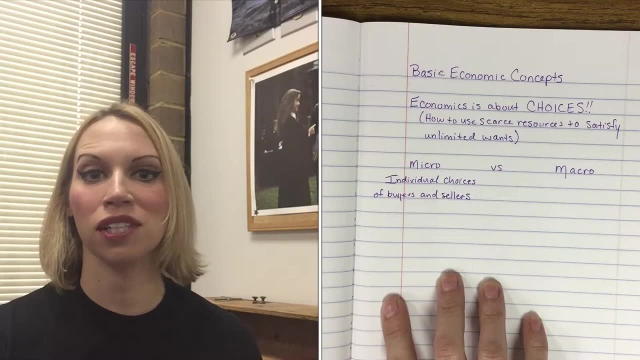 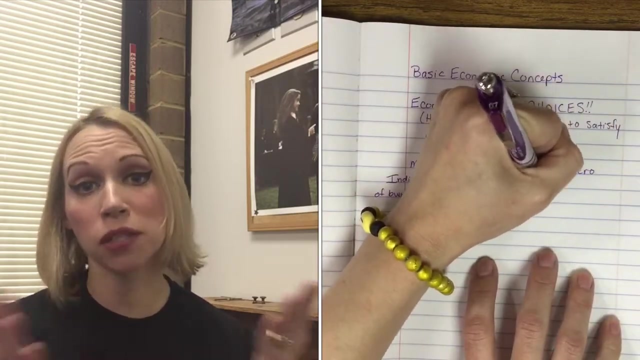 to figure out how customers can get the best deals. We're going to figure out how businesses can maximize their individual profits and all of those things are practical things to know how to be able to do With macroeconomics. we're going to be talking about things on a bigger scale. 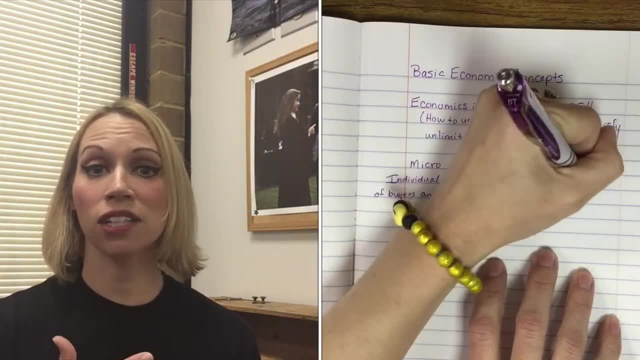 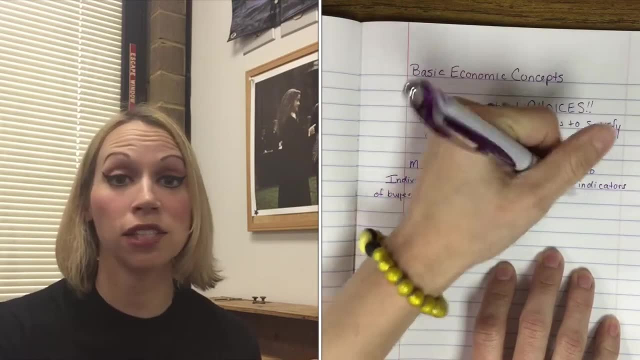 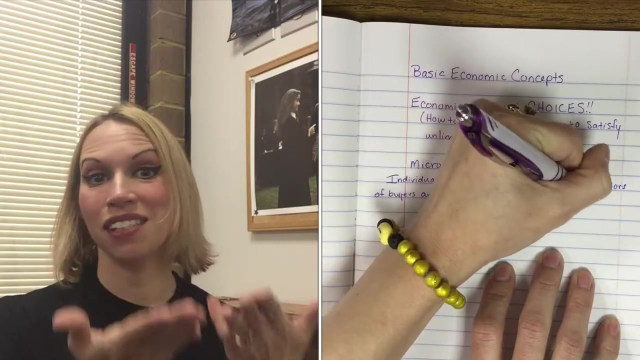 So things that concern the entire nation, like a country's GDP, how productive is a country? is that country's currency appreciating or depreciating? We're going to talk about foreign exchange. We're going to talk about inflation, and if the price level of things is getting higher, or 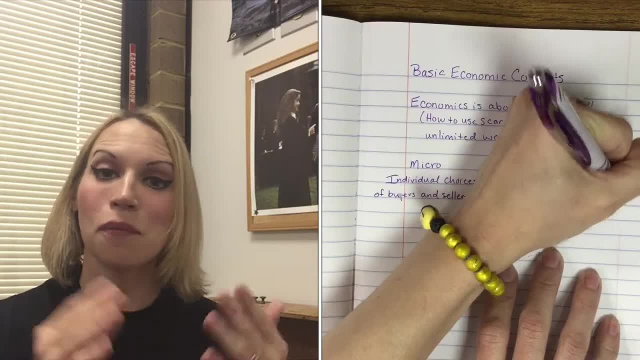 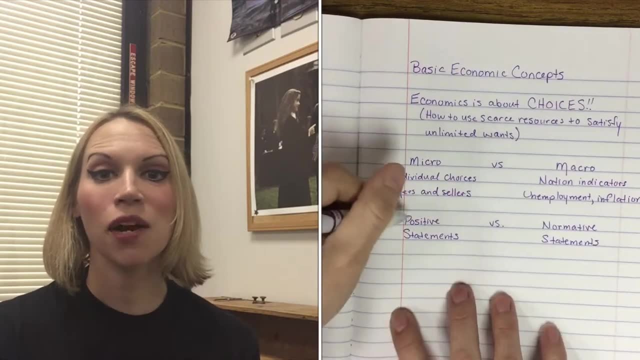 lower, and we're going to talk about unemployment as well. So macroeconomics deals with bigger things that concern the whole entire country or the whole entire economy. Now, what do economists actually do? Well, when they're hired by businesses or by a government, then what they tend to do is: 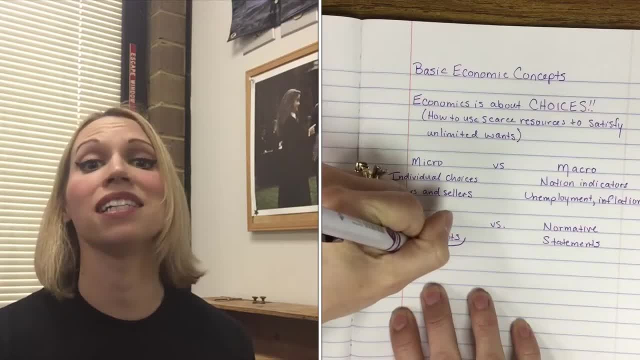 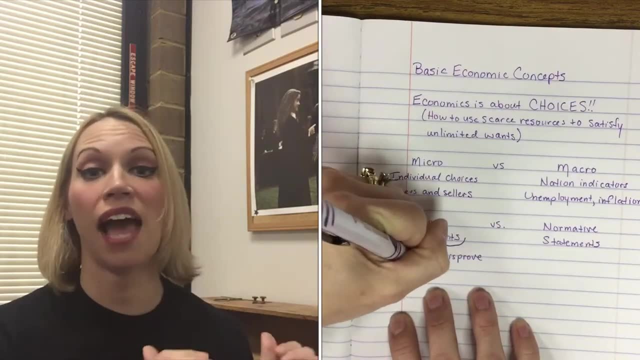 study data and then give advice based on what they see in that data. A lot of times they're studying sales data and they're using positive statements to describe how things actually are. So an economist would actually use positive statements when they're looking at the quarterly sales data to figure. 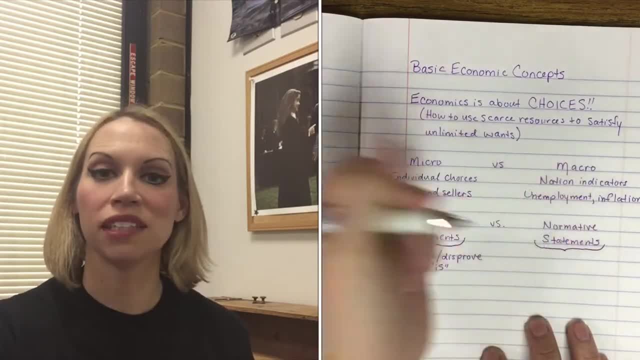 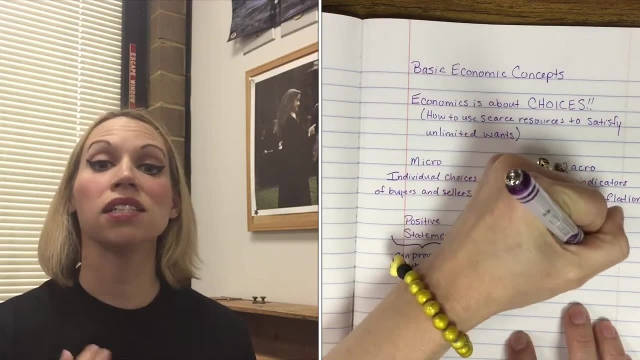 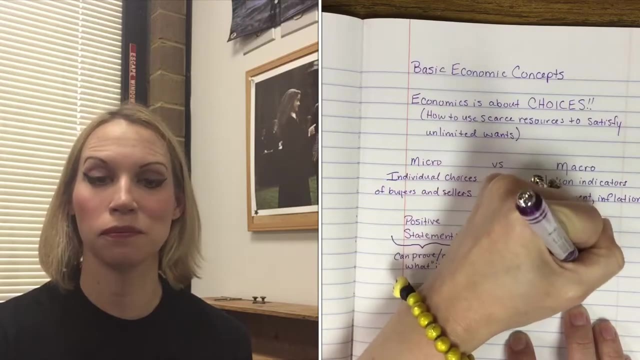 out how sales actually are for that company And then, based on that information, they're going to use normative statements or statements of opinion to talk about what they think the company should do to maximize its profits or to increase its sales. now for us in our 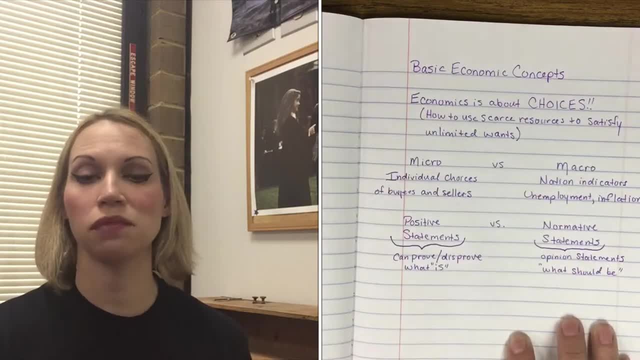 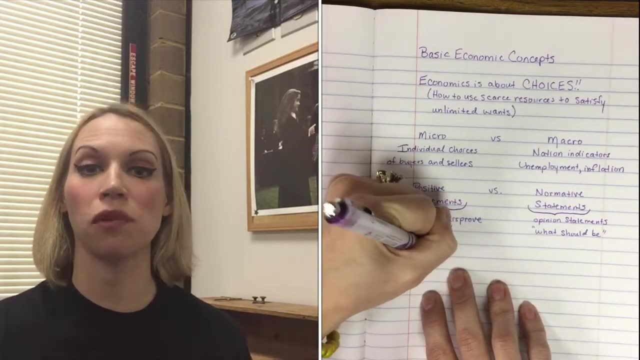 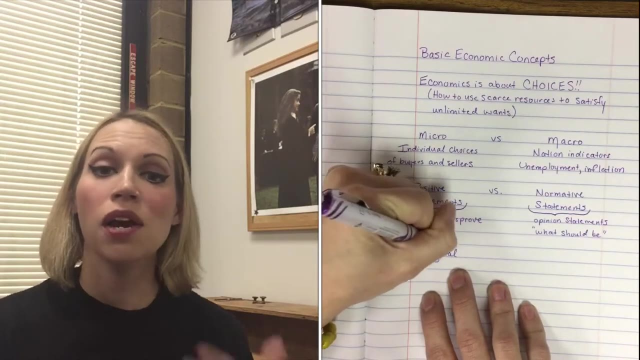 everyday life. we're always, constantly making choices. we make multiple choices every single day and most of us don't realize it, but we instinctively use a process called marginal analysis. you probably know this as weighing the pros and cons of something. in economics, the word marginal always means something. 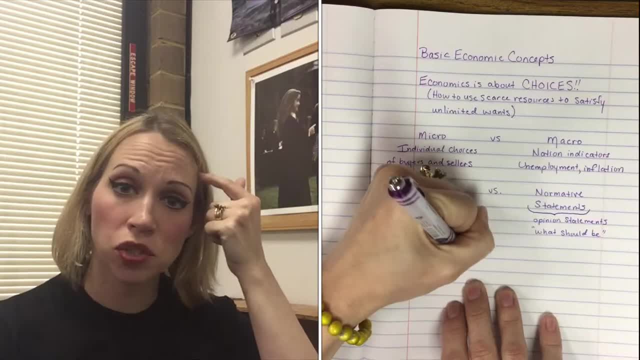 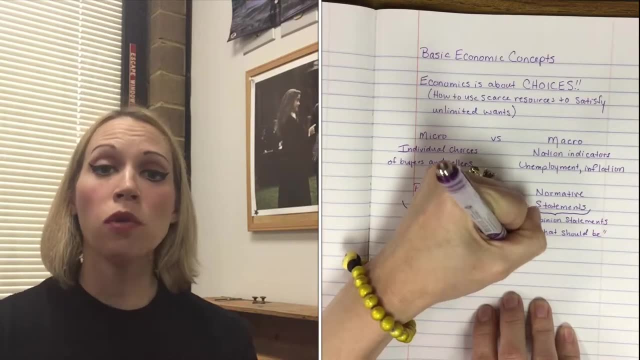 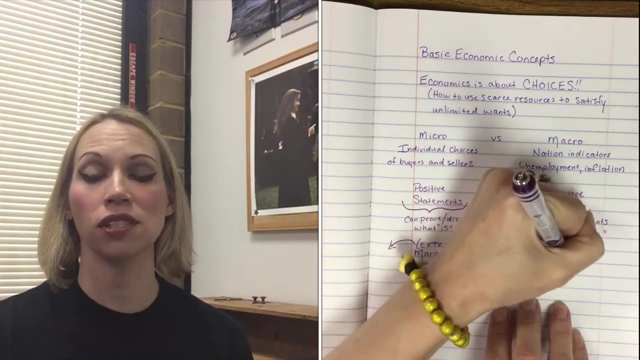 extra or something additional. so when you think of marginal, think of extra or additional, like how margins on the side of a page are extra or additional space. when we do marginal analysis, we're weighing the extra benefits of something versus the extra cost of that action. now, of course, if the cost outweigh the, 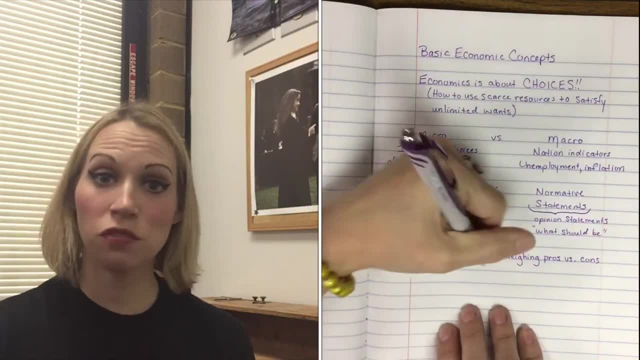 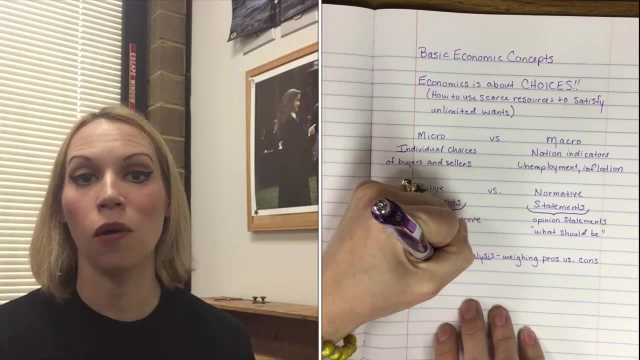 benefit, we probably won't do that action. but if the benefits outweigh the cost, we will probably do that instead proceed with that action. so marginal analysis is simply what a lot of people call weighing the pros and cons of something, and that's how we make our. 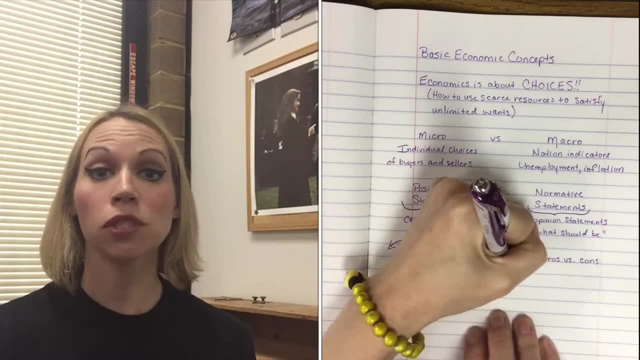 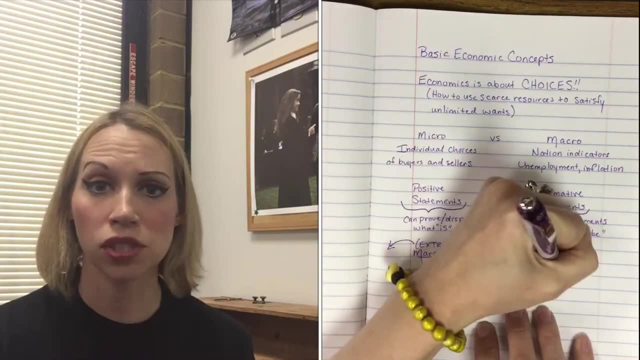 choices now. anytime that we make choices, we're trying to make the best decisions we can for ourselves, given the information we have, and that's called acting in our own rational self-interest. and most of us, we assume, are trying to make the best decisions for ourselves, given the information we have. whether 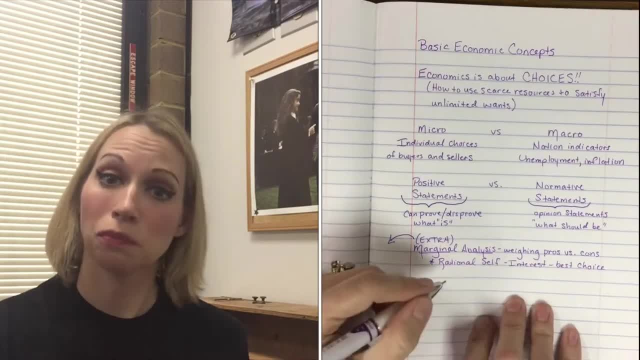 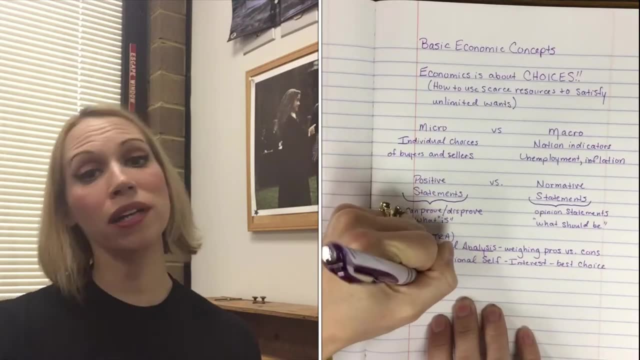 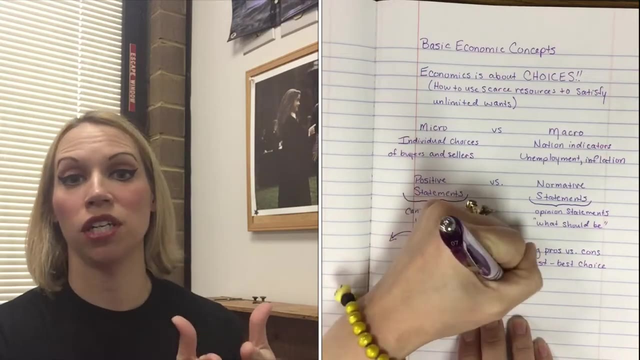 you're trying to decide what college to go to or what car to buy, basically based on the information you have. you're going to try to make the best decision you can. anytime you make a choice, there are always alternatives that you did not choose, and those are known as trade-offs. now the next best alternative, or your. 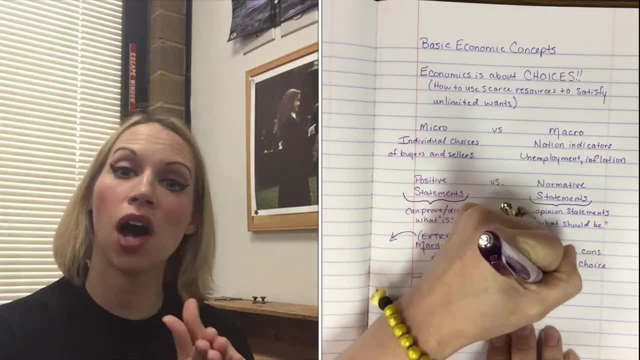 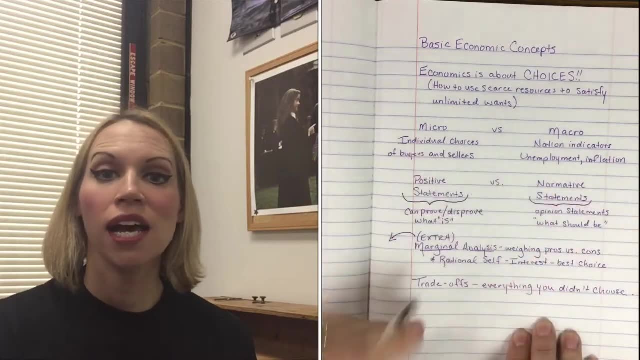 second best choice is known as something specific, called opportunity cost. opportunity cost is that next best alternative that you did not choose, and it does not have to be a dollar value just because it has the word cost in it, maybe what you're giving it a chance to do so. 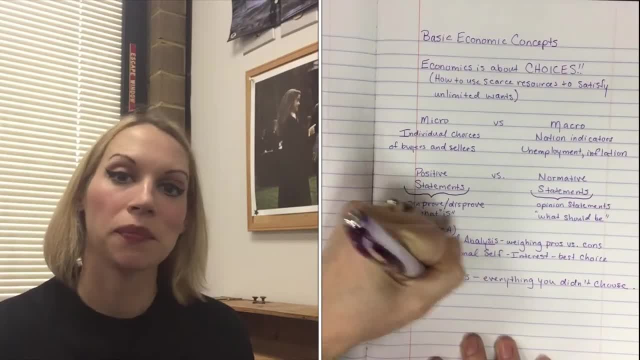 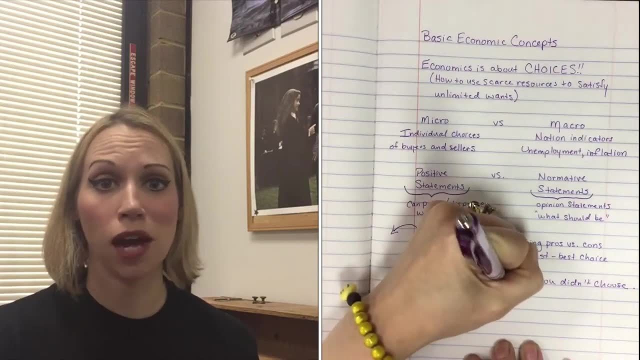 So the next best choice is the experience of something. for example, if you've ever gone to a restaurant and you're with a group of people, sometimes you might have difficulty looking at the menu and all the different options, trying to decide what it is that you want to eat. I know that's me. I'm always the last. 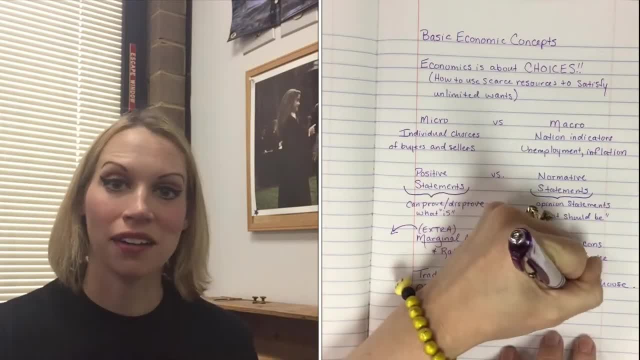 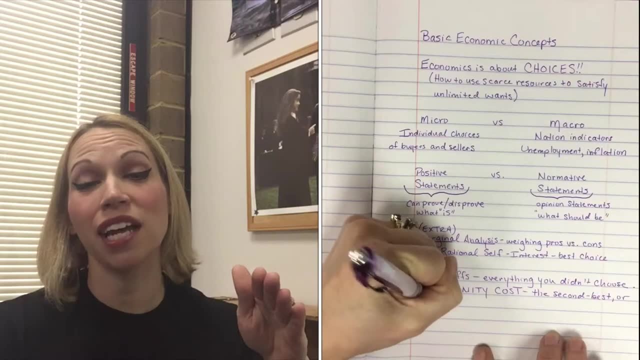 to decide what I want to eat. eventually I get it narrowed down and eventually I make my decision, even though I chose the chicken pasta. maybe, if I hadn't chosen that, I would have chosen the hamburger, or I would have chosen the sauce, the hamburger, or I would have chosen the sauce. 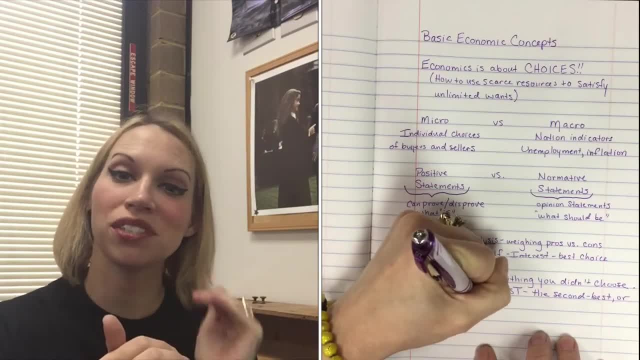 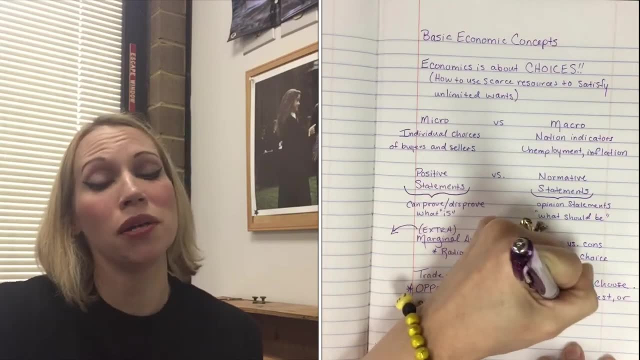 or I would have chosen the sauce, or I would have chosen the sauce- salmon, right. whatever is your second best choice. that's known as your opportunity cost. so even though I got the chicken pasta- and it was delicious- I also did miss out on the yumminess and the experience of the other food that I